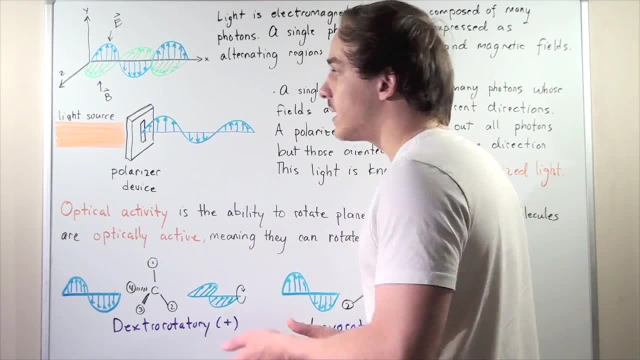 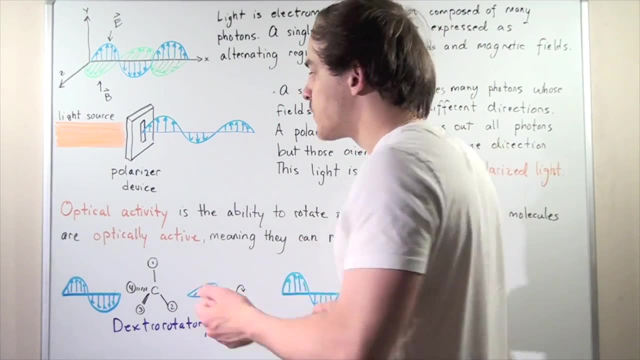 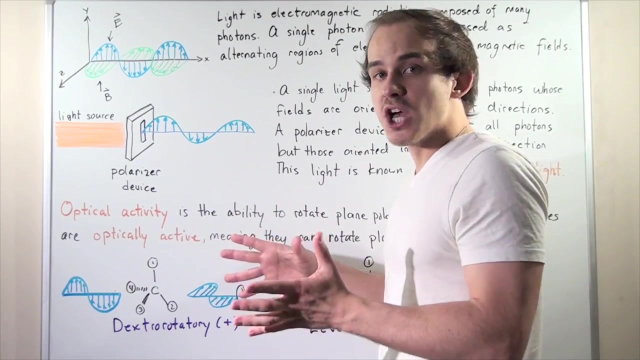 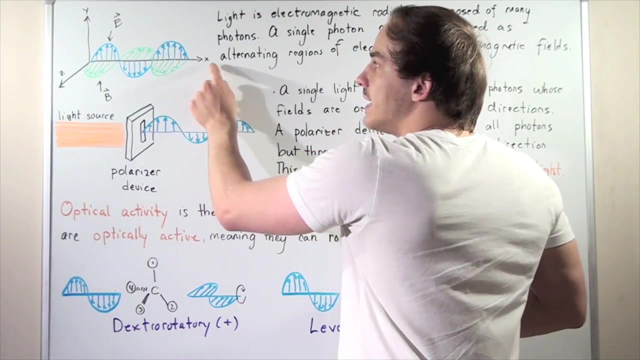 light, our electromagnetic radiation, our photons, And that's shown here. Now, all these photons have fields oriented in different directions. What this polarized device does is it polarizes the light, screens out all different types of directions of fields and only leaves the ones that point in this direction. Let's say it's. 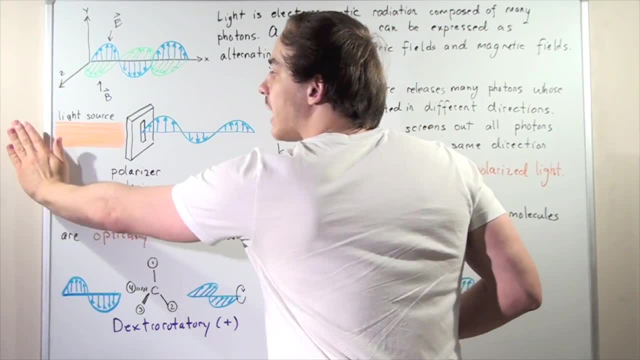 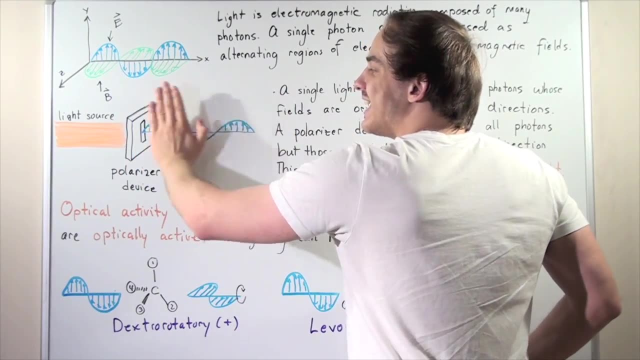 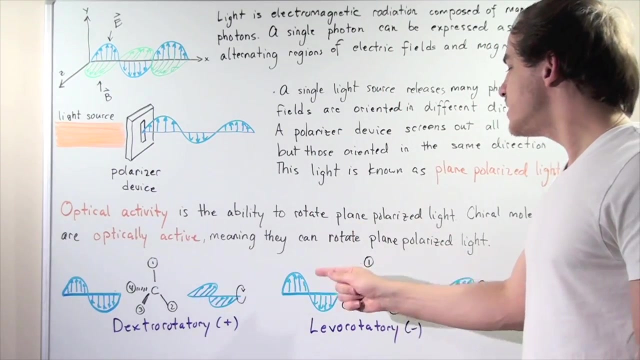 along the x-y axis. So once light comes through our device, only electromagnetic radiation pointing in one direction exists along the x-y direction. Now optical activity is the ability to rotate plain polarized light. Now there are certain molecules or compounds that exist that exist along the x-y axis. Now optical activity is the ability to rotate plain polarized light. Now there are certain molecules or compounds that exist. 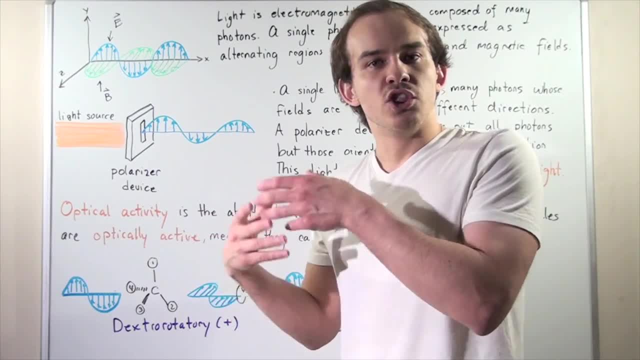 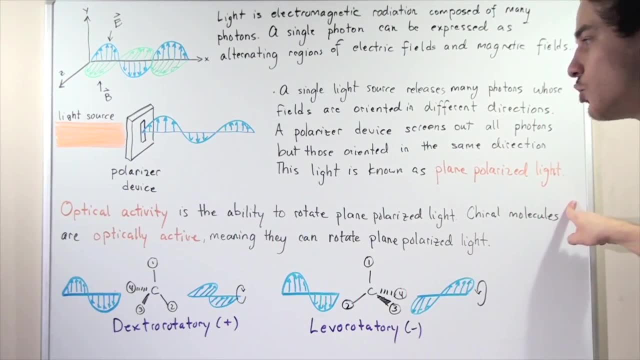 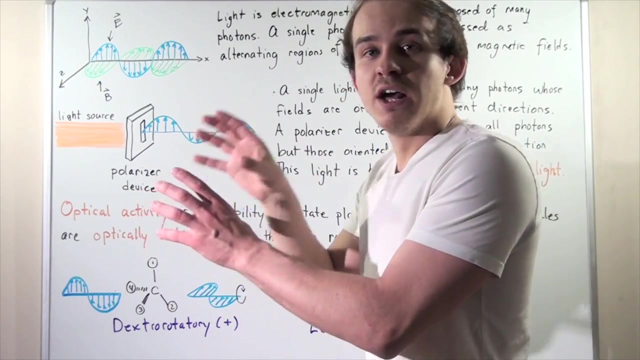 that when you shine light on those molecules, those molecules reflect the light and rotate that light. And in fact chiral molecules are optically active and that means that they rotate plain polarized light. So if you take this type of polarized light and you shine it on a chiral molecule, that molecule 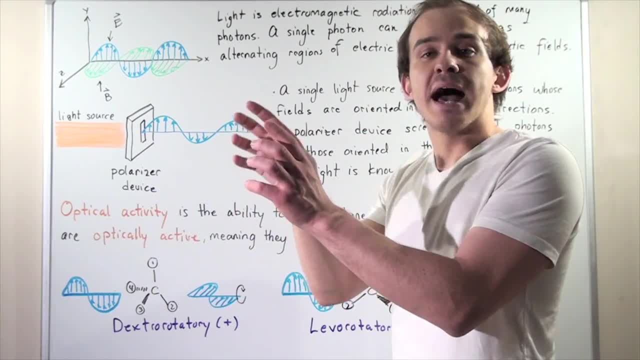 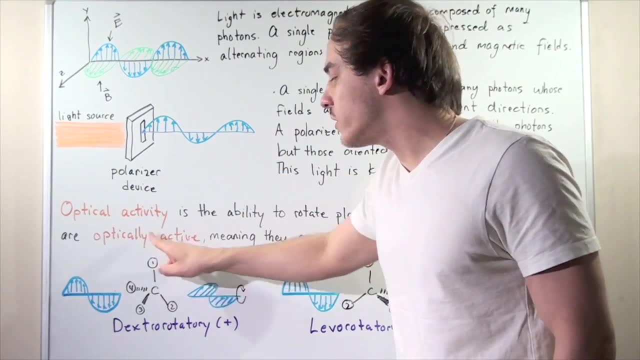 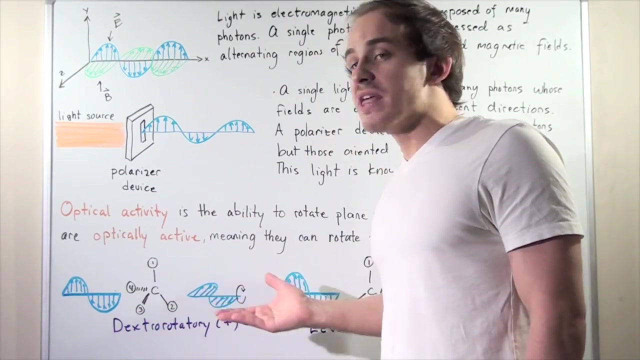 will rotate that light a certain amount of degrees. now one important difference exists. so let's suppose we have the following important chiral molecule. and this chiral molecule has a mirror image, right, because if it's chiral, that means there exists a second enantiomer, that is: 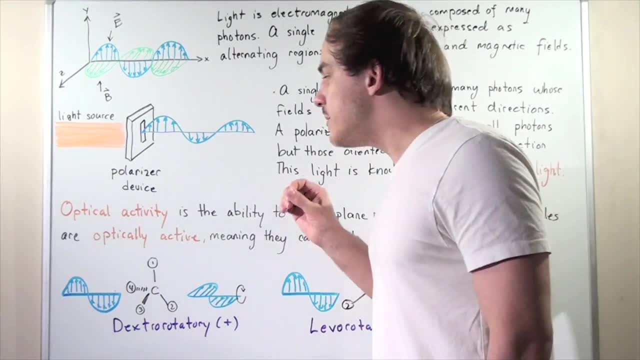 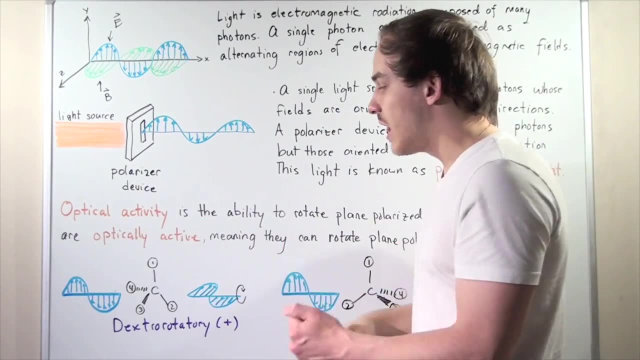 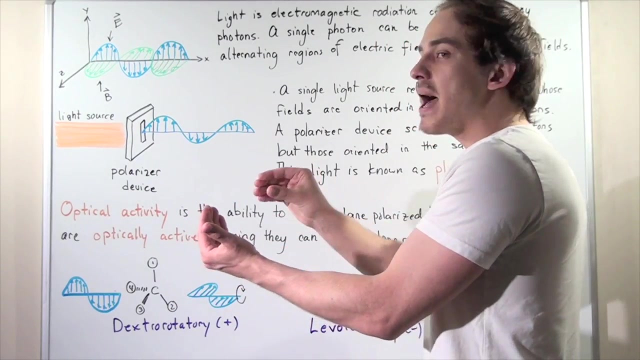 the mirror image shown here. now, what do we mean by optically active? so if we take this plane polarized light and we shine this line on our molecule, this molecule will rotate, that like a certain amount of degrees and let's say this anatomy, for instance, rotates our life. 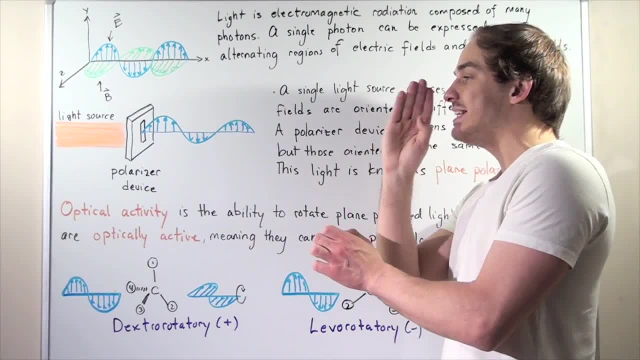 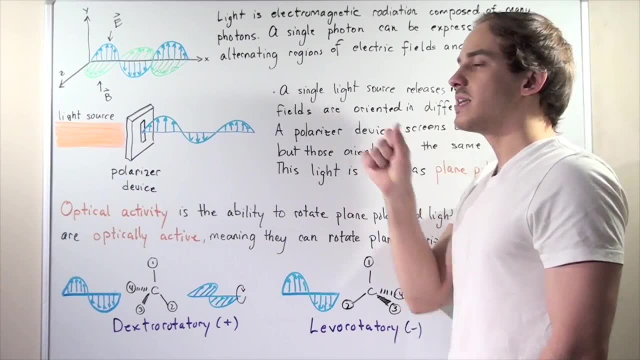 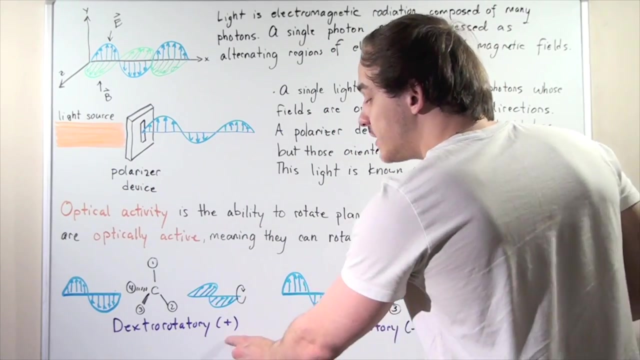 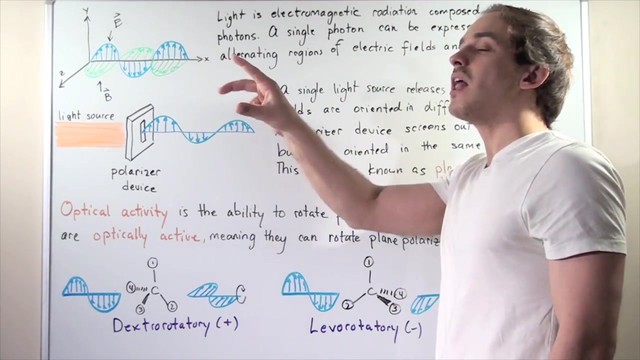 clockwise. so if we're looking at our molecule, at the incoming light, when the light comes through the molecule, the molecule will rotate it clockwise. and if your rotates it Francia, as saying a line below the right hand side, corresponding to the order of니 Clockwise, we call it dextrorotatory and we give it a positive sign. So positive means dextrorotatory. that means the light is rotated clockwise as we're looking at the light, as it's coming in.